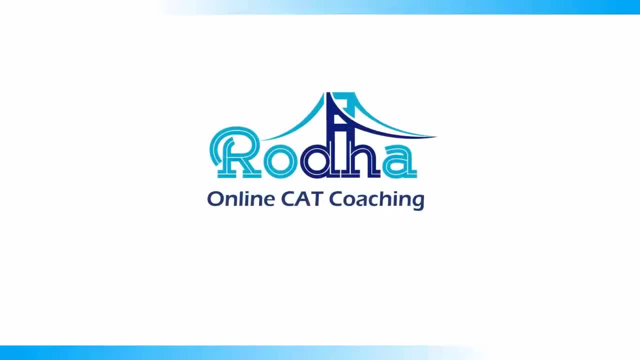 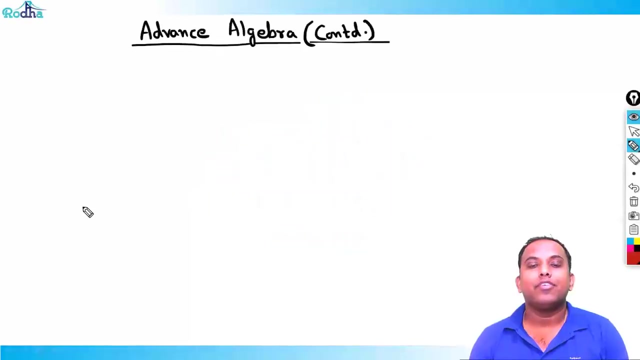 Hi everyone, my name is Ravi Prakash and welcome to the next class of Advanced Algebra. So again, we will discuss some very important concepts and questions here. The first one will be: if 2 raised to x is equal to 3 raised to y is equal to 6 raised, 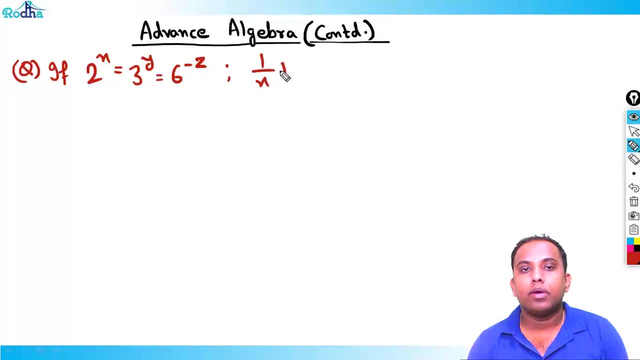 to minus z. Okay, what is the value of 1 by x plus 1 by y plus 1 by z? is the question right? So one similar question in CAT was asked in CAT 2015,. okay, And this is very common for SSC also, kind of examinations. okay. 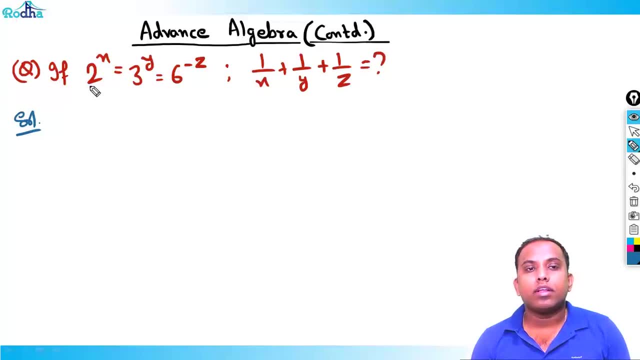 So we'll learn how to solve this kind of question right Now. see if these are like the three terms here: 2 raised to x equal to 3 raised to y, equal to 6 raised to minus z. So what we should do is first, is we should equate all to k. 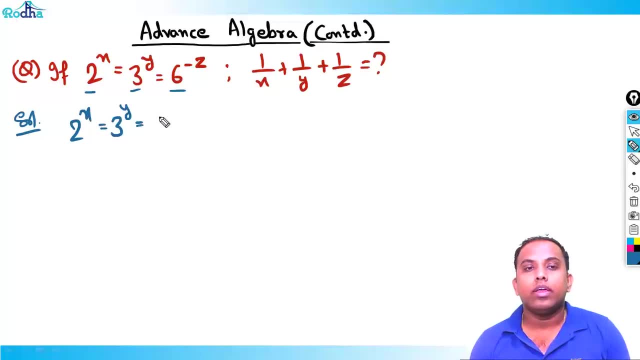 2 raised to x, equal to 3. raised to y, equal to 6. raised to minus z, equate to k. Okay, so what will happen? right? The basic rule is actually: if a raised to m is equal to b, then a is equal to b raised. 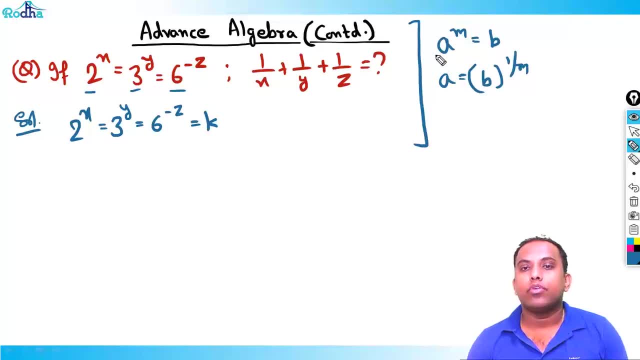 to 1 by m, Right. This you know. if a raised to m equal to b, then a is equal to b raised to 1 by m. Both right sides. we take mth root, So b raised to 1 by m right. 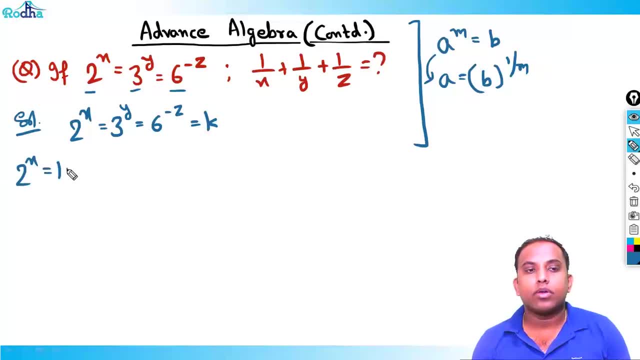 So simply here also: 2 raised to x is equal to k, right? So 2 is equal to k raised to 1 by x, right? Then 3 raised to y is also equal to k, So 3 is equal to k raised to 1 by y. 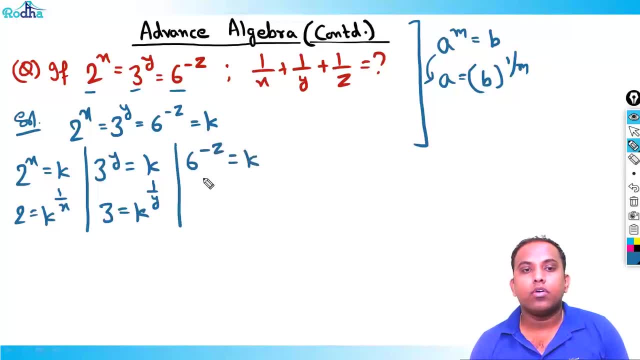 Then 6 raised to 1 by y is equal to k, Right. Then 6 raised to minus z is also k. okay. Then 6 raised to minus z is also k. Then here 6 is equal to k raised to minus 1 by z. fine, fine, okay. 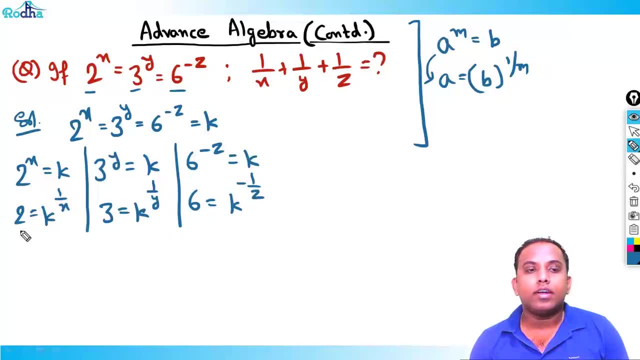 Now. so we got this results here, right? So now we have to see here that this number here is 2,, this number here is 3, and this number here is 6, right, So we know that 2, I can relate, I can correlate these 3 things as 2 into 3- is equal to 6, okay. 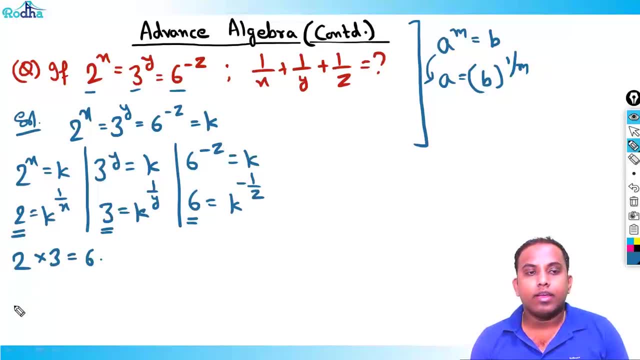 So if 2 into 3 is equal to 6, then k raised to 1 by x into k raised to 1 by y is equal to k raised to minus 1 by z, correct? I can write this as now. this will turn to what. 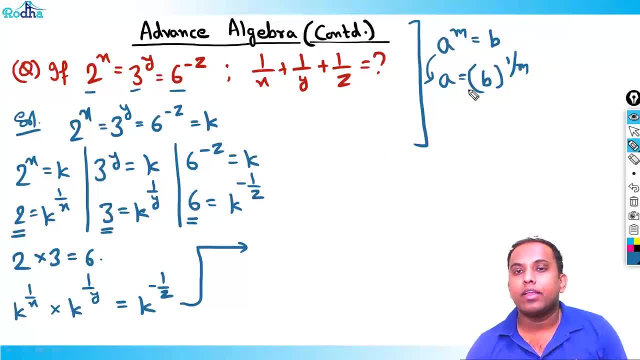 This will turn to now, since the bases are same. right, So we know it. So we know again that a raised to m into a raised to n is equal to a raised to m plus n, right? So here also this base will add, so I can write: k raised to 1 by x plus 1 by y is equal. 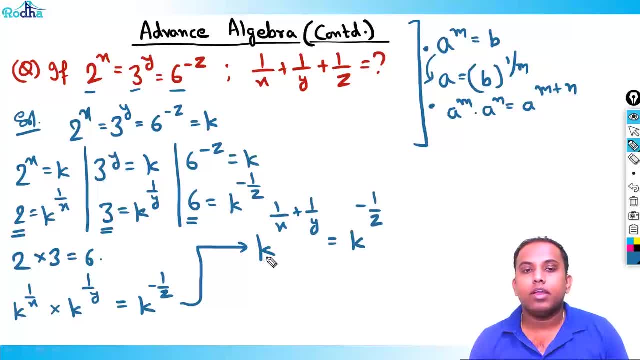 to k raised to minus 1 by z, correct. And then we also know that if a raised to m is equal to a raised to n, then m is equal to okay, sorry. Then m is equal to n, okay. So m is equal to n here and when m is equal to n, knowing that m is equal to n, knowing 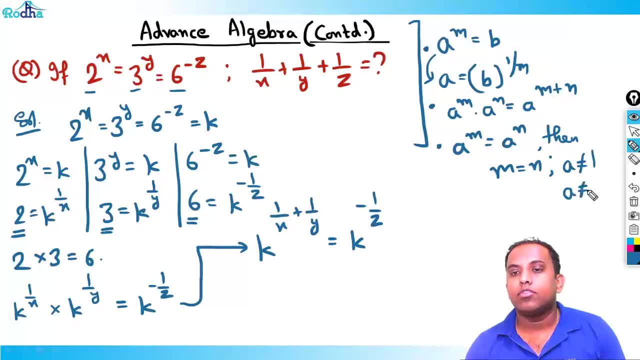 that a is not equal to 1 and a is not equal to 0, obviously right, Because each term a should not be 0 here, because if a is 0, 0 raised to something will not be valid. right, For m may not be equal to n, because 0 square equal to 0 cube okay. 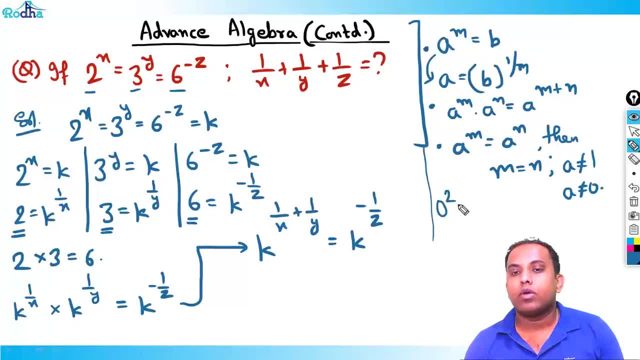 What I'm saying is: Suppose 0 square is equal to 0. Okay, So 0 square is equal to 0 cube. So both are 0, 0, right. 0 equal to 0. That doesn't mean that 2 equal to 3, right. 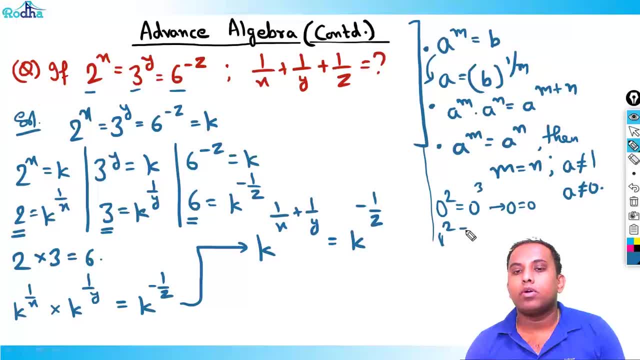 Or or same thing for 1. also, 1 square may be equal to 1 cube. that means 1 equal to 1.. That doesn't mean that 2 equal to 3, right. So it is not valid for 0 and 1. basically, right. 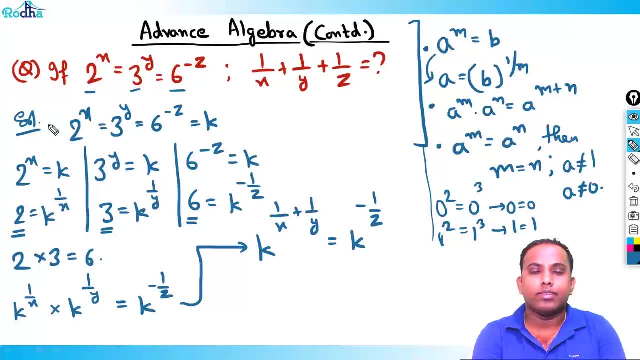 So here obviously it is not this: x y z are not 0, right, So 1 by x plus 1 by y, equal to k raised to minus 1 by z. okay, Or yeah, x y z. 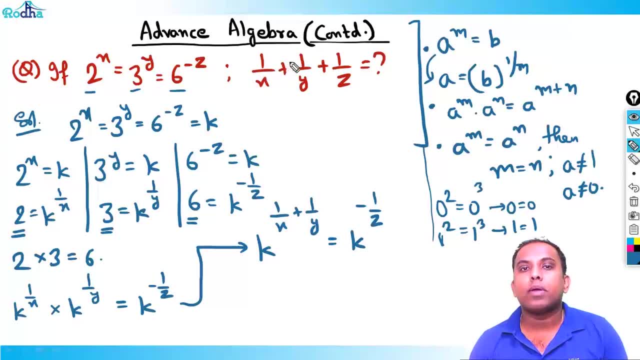 They are not 0 because I need to find a value of 1 by x plus 1 by y plus 1 by z. okay, So the denominator cannot be 0, denominator cannot be 0, this cannot be 0, right. 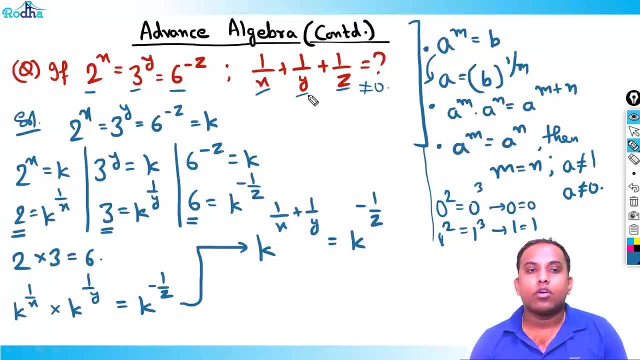 So x y, z are not 0s here, obviously okay. So x y, z are not 0s here. And since they are not 0s here, there are some values. So 2 raised to some value will give some positive value, right. 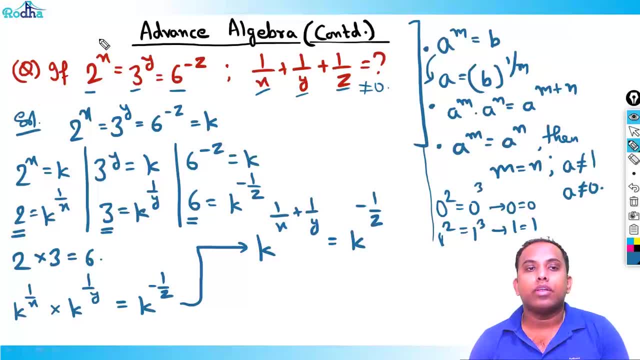 They are not 1, also right, Obviously, since they are not 0, so we'll get a equal to 1.. That means we'll get this equal to 1.. Okay, So if x is equal to 1, 2 raised to x will be equal to 1 only when 2 raised to 0. 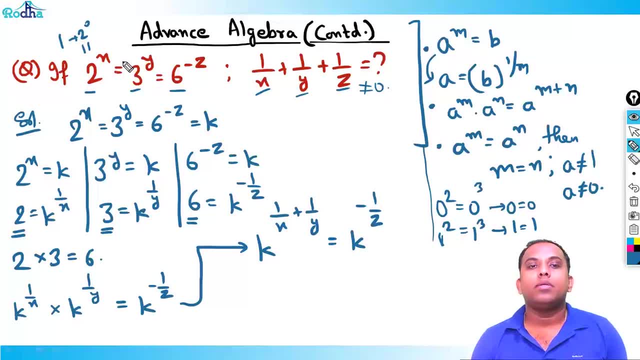 It becomes 2 raised to 0,. right, Since x is not equal to 0,, it doesn't become 2 raised to 0, also, right? So these two things are automatically excluded here. okay, Fine, So I can simply now write: okay, so 1 by x plus 1 by y equal to minus 1 by z. 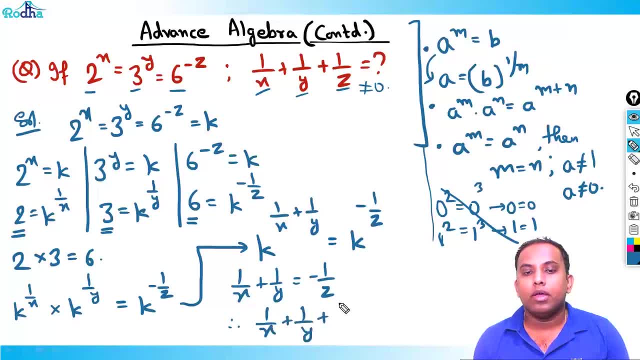 Therefore, 1 by x plus 1 by y plus 1 by z is equal to 0.. That's the answer. okay, This is the answer. So the question was: what is the value of 1 by x plus 1 by y plus 1 by z? 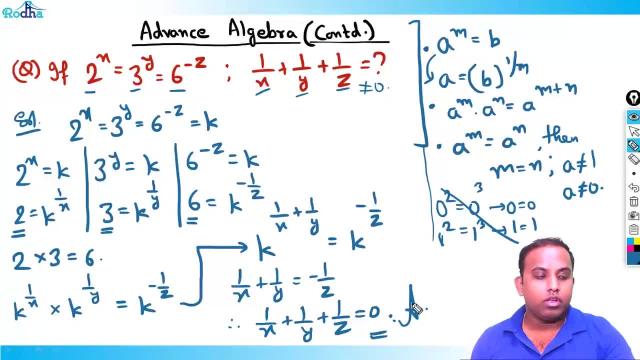 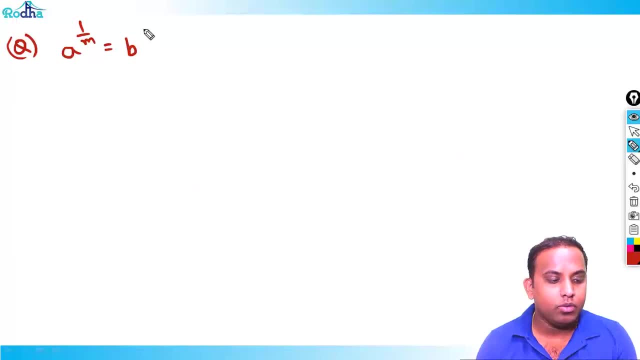 Answer is 0.. Answer is 0.. Next question we'll see. Next question is a raised to 1 by m is equal to b. raised to 1 by n is equal to c raised to 1 by p. Okay, c raised to 1 by p. 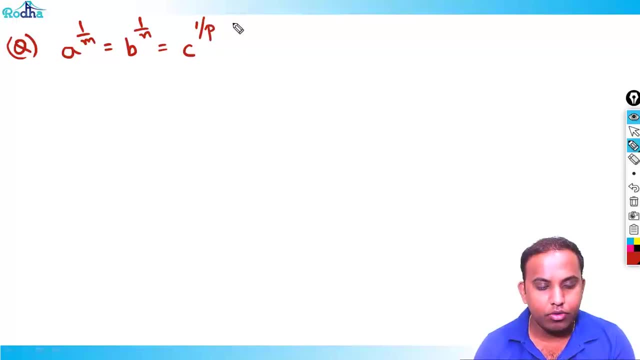 Fine, So you need to find the value. Ok, You need to find the value of given that a b c is equal to 1.. Okay, If a b c equal to 1, you need to find the value of m plus n plus p. 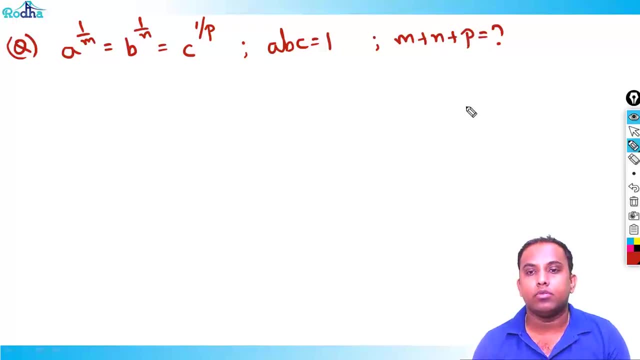 m plus n plus p, you need to find a value. okay, And let's solve it again. So a raised to 1 by m is equal to b, raised to 1 by n, equal to c. raised to 1 by p, Then a b c equal to 1 by n. 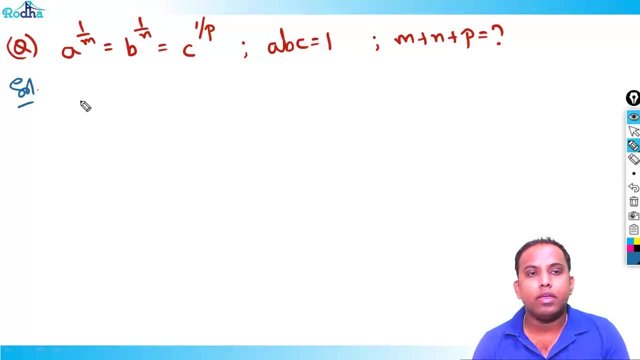 So again, it's the same as we learned earlier: a raised to 1 by m is equal to b. raised to 1 by n is equal to c. raised to 1 by n. raised to 1 by p equate all to k, right. so if this is, all are equal to k. so now a raised to 1 by m. 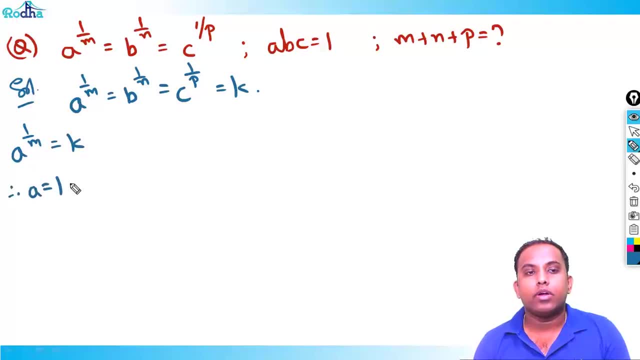 is equal to k. therefore, a is equal to k raised to m. okay, b raised to 1 by n is equal to k. so b is equal to k raised to n. right? and c raised to 1 by p is equal to k. okay, c raised to 1 by p is equal to k. therefore, c is equal to k raised to p. right, okay. so what we know. 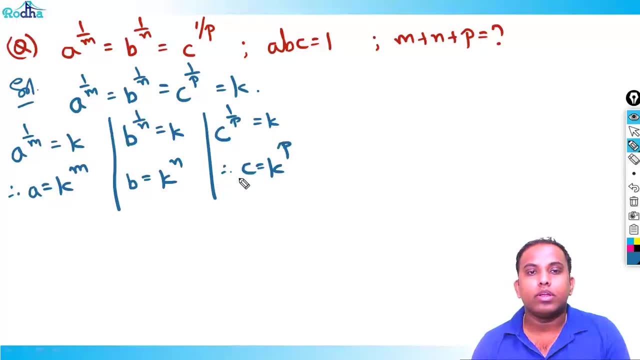 now here is a, b, c equal to 1, so multiplying this we'll get this one right. so since a into b into c is equal to 1, therefore k raised to m into k, raised to n into k, raised to p, is equal to 1. 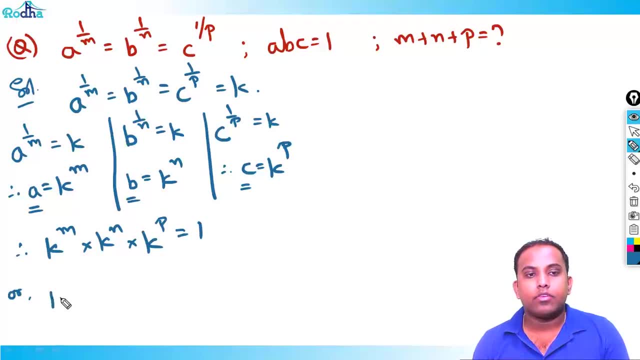 correct. so now k raised to m plus n plus p is equal to 1. so 1 can be written as k raised to 0, right 1 can be written as k raised to 0, again same for that. so since these two are equal, so i'm going. 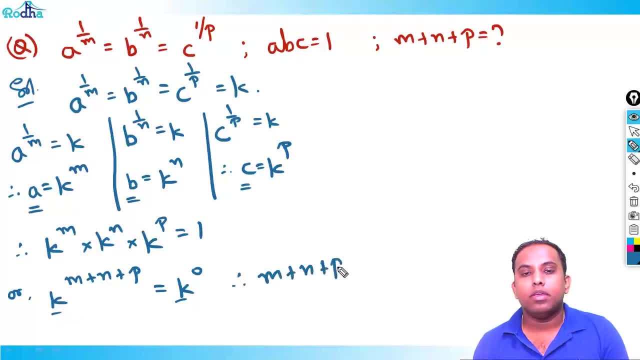 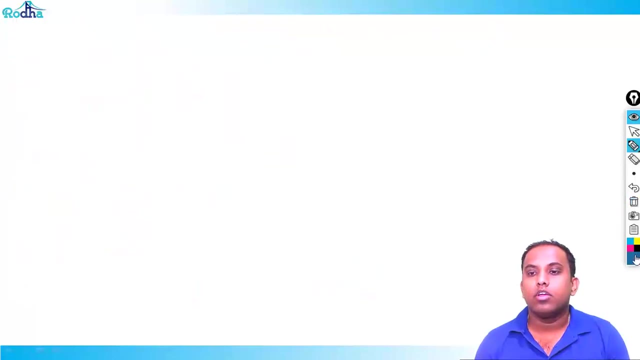 to write: therefore, m plus n plus p is equal to 0. that's the answer for this question, correct, right? everybody's clear now, okay, just this kind of questions, fine, okay. so next question is now: if x is equal to 2 plus 2, raised to 2 by 3, minus 2 raised to 1 by 3, okay, then find the value of x cube minus 6 s square. 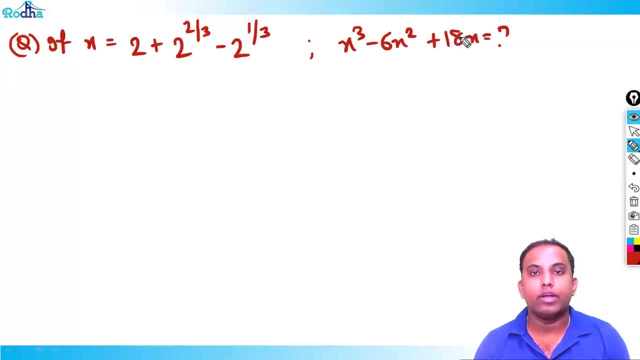 plus 18 x is equal to what we need to find the value of x cube minus 6 s square plus 18 x is equal to what? now see again a very good question. so let's find the value of x cube minus 6 s square. 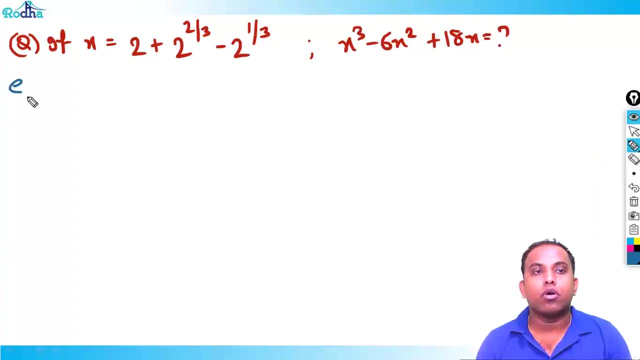 plus 18, x. i need to find the value and this is given right. so what we'll do, basically, i need to observe here is: i need to observe here is: here the term required is x, cube, x, square and x. okay, so decreasing power of x, x, cube, x, square and x. and here here it is: 2 raised to 2 by 3. 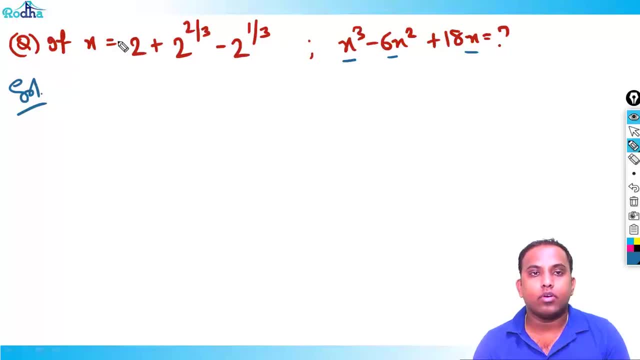 and 2 raised to 1 by 3, right, and here it is x, okay. so what I can do here right now is I can write: x is equal to, okay, sorry, x minus 2 is equal to 2 raised to 2 by 3 minus 2 raised to. 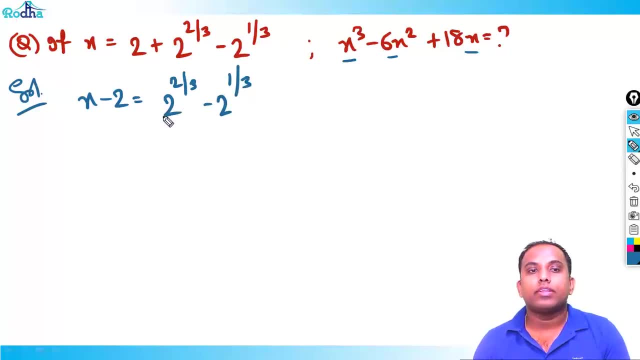 1 by correct. so now, if it is right, if it is like this, so now we can observe it, we need this term, so we have to cube both sides. right, so we have to cube both sides. okay, to get this. 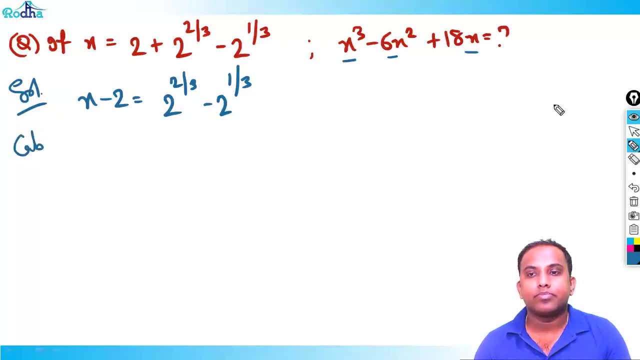 term right, so we'll cube both sides. so cubing should write here that cubing both sides, cubing both sides. x minus 2, whole cube is equal to 2 raised to 2 by 3 minus 2 raised to 1 by 3. 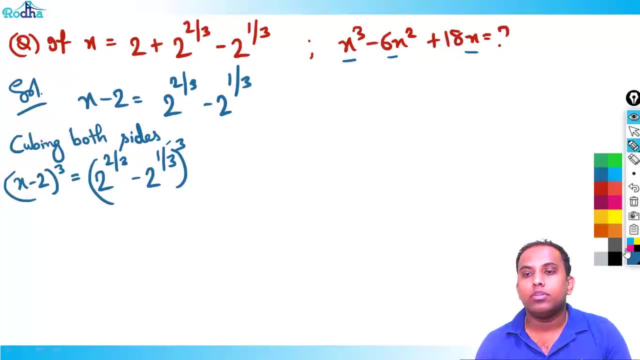 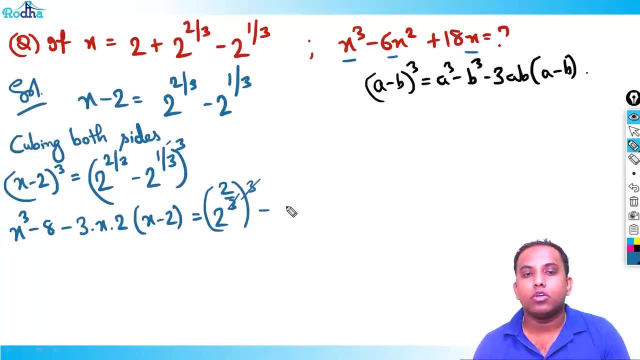 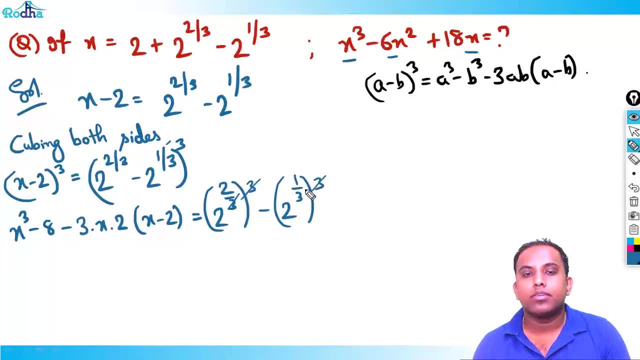 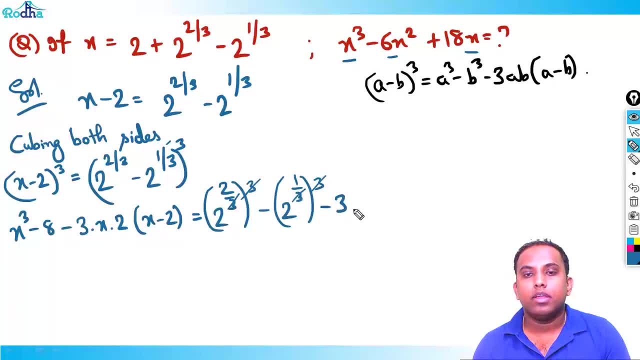 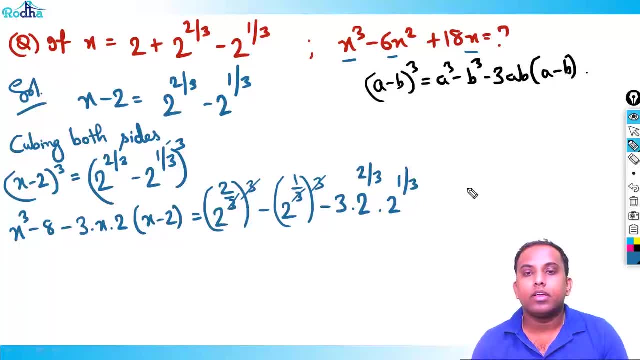 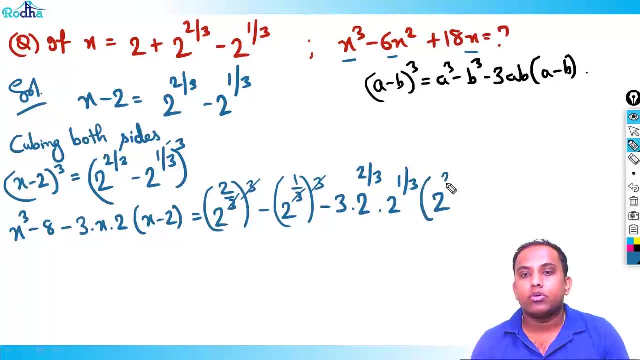 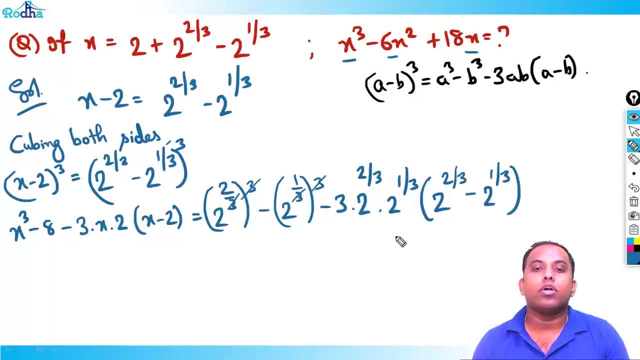 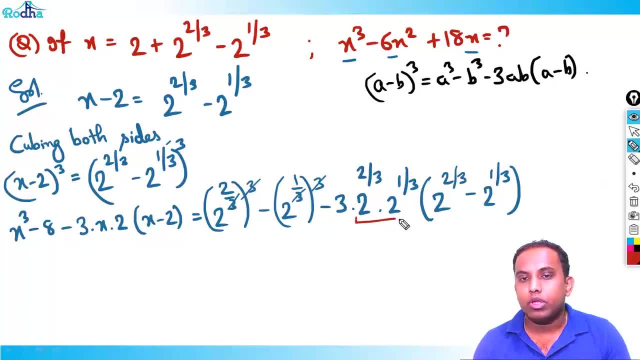 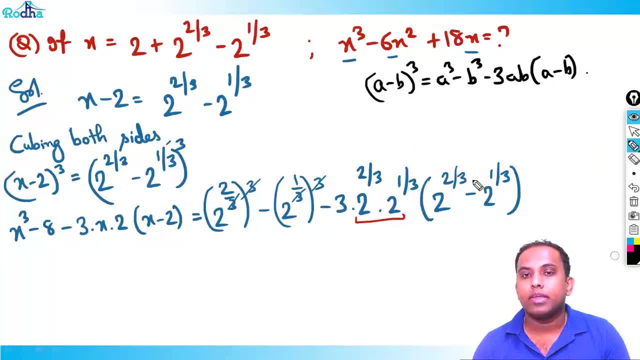 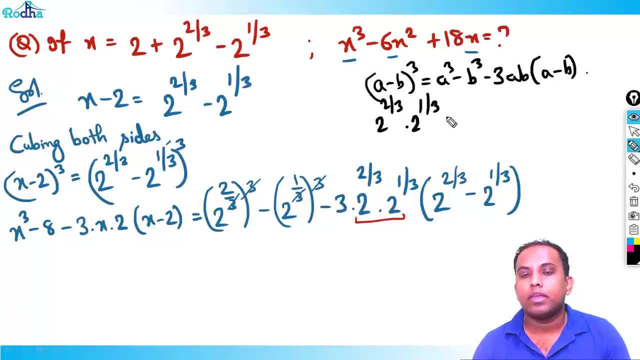 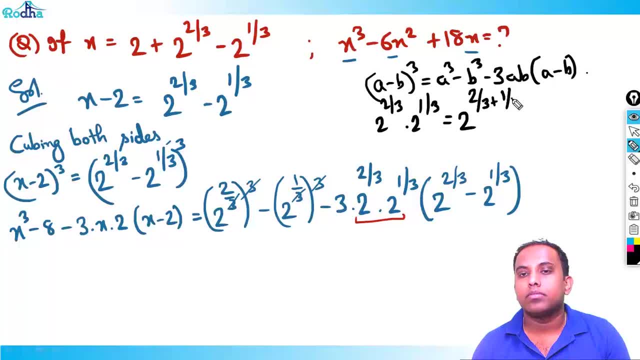 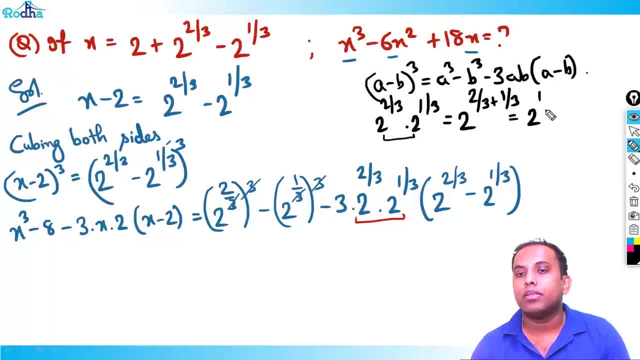 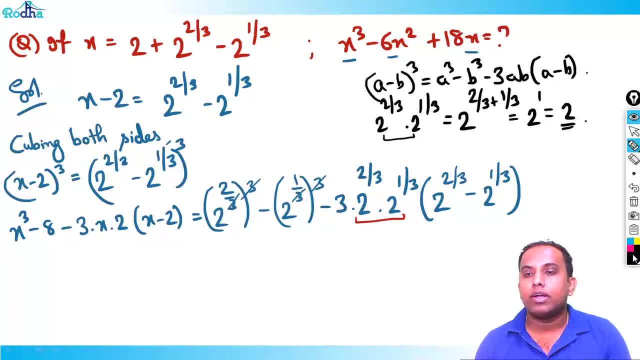 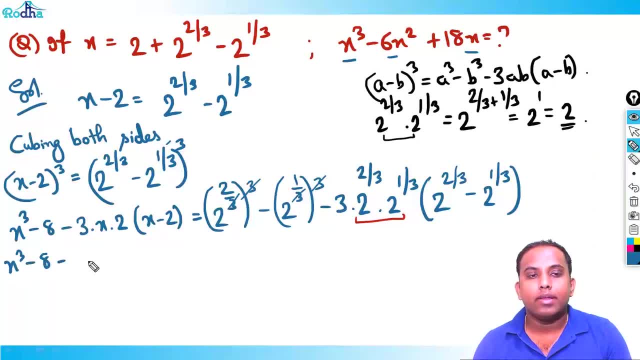 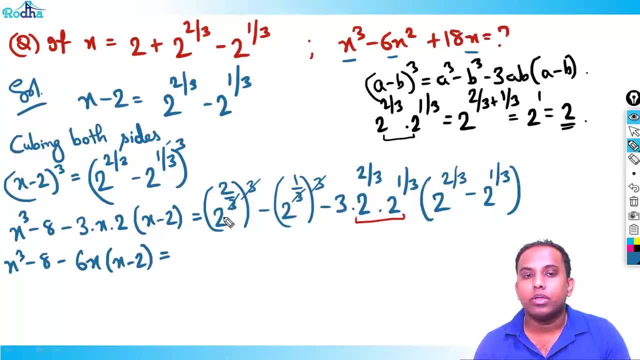 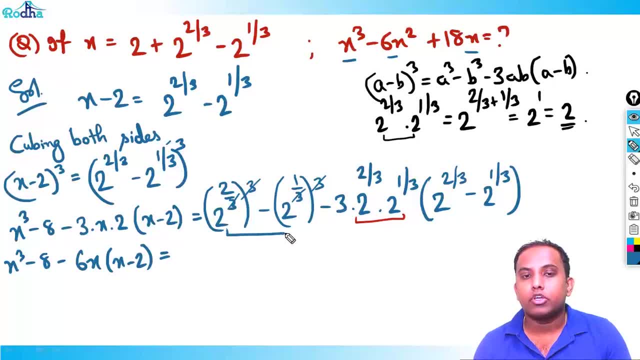 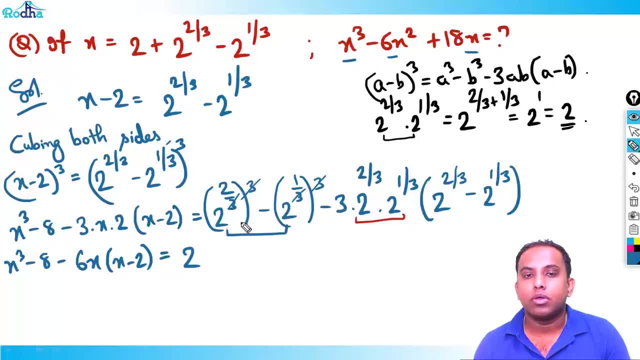 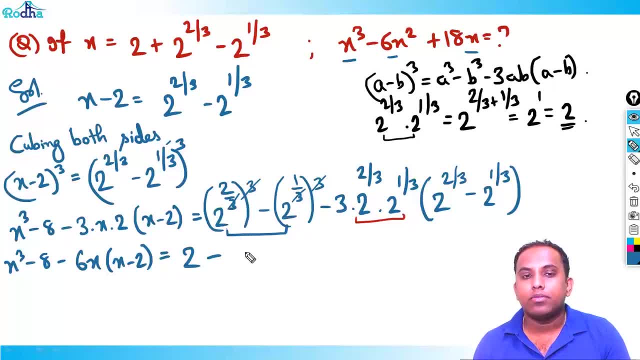 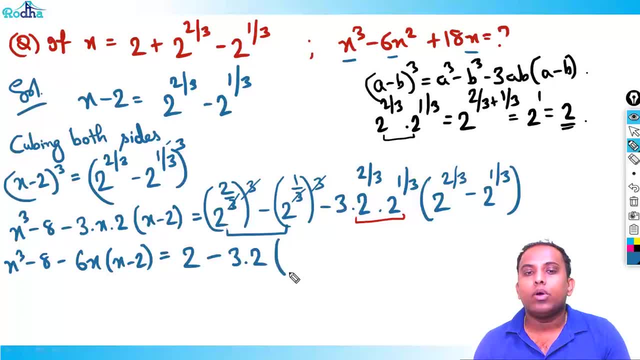 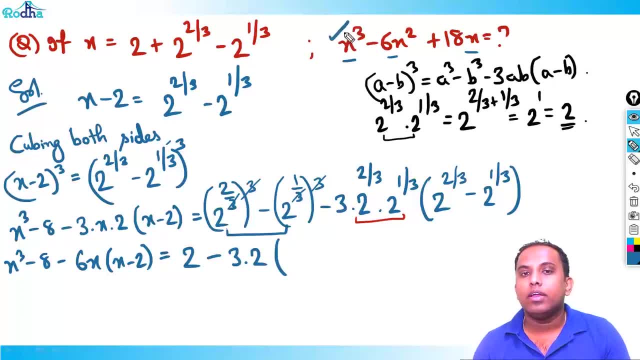 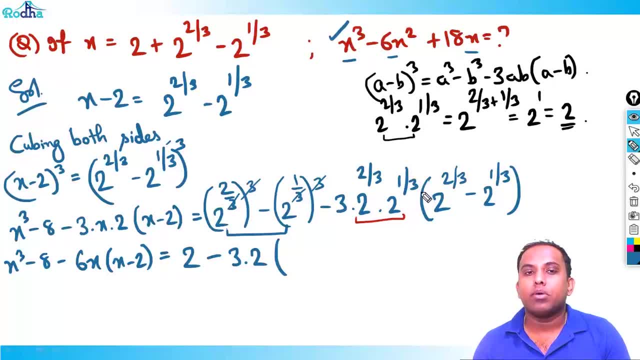 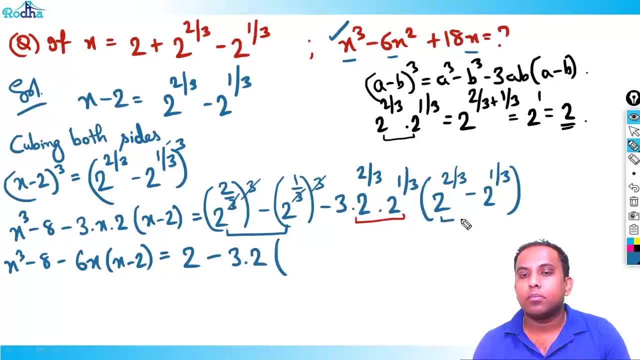 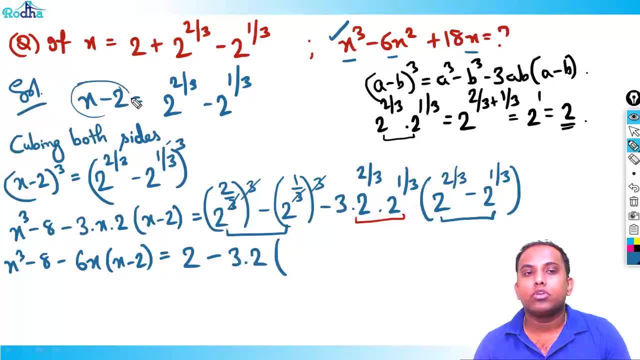 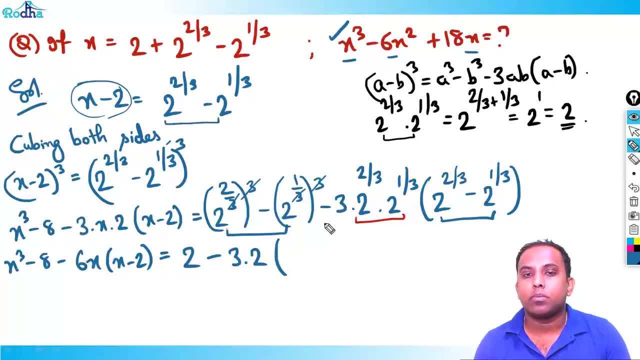 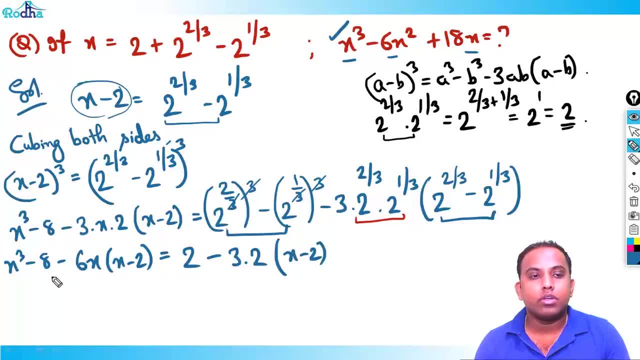 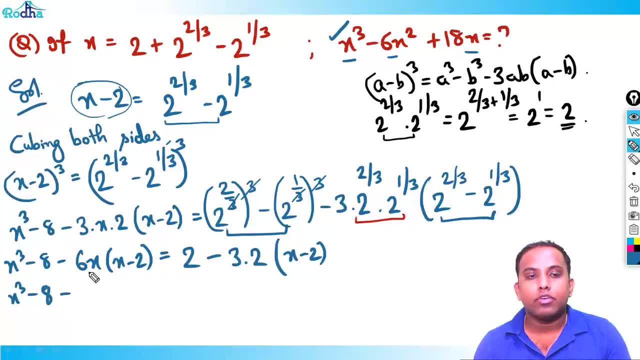 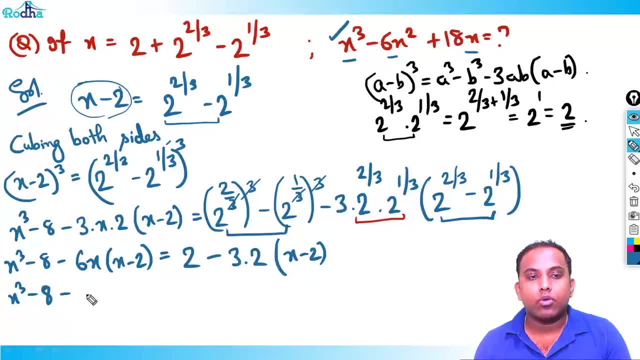 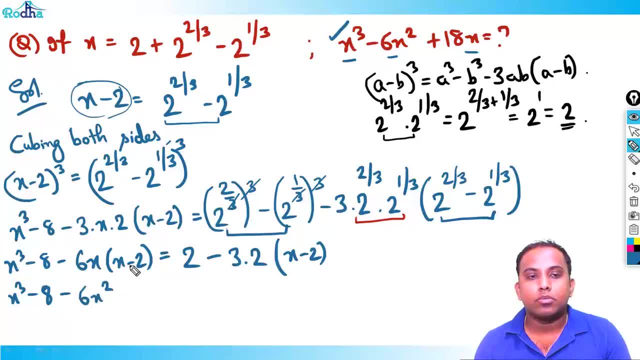 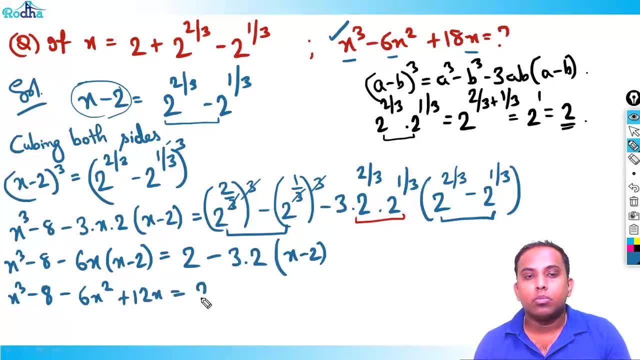 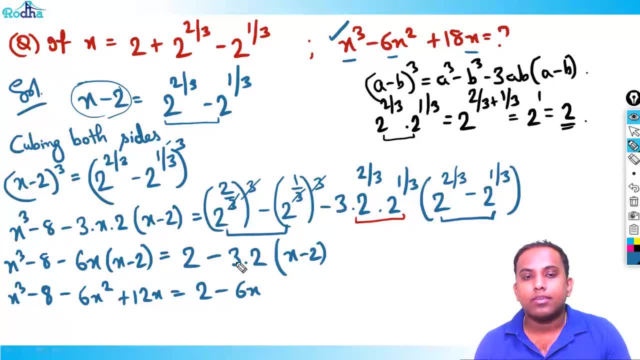 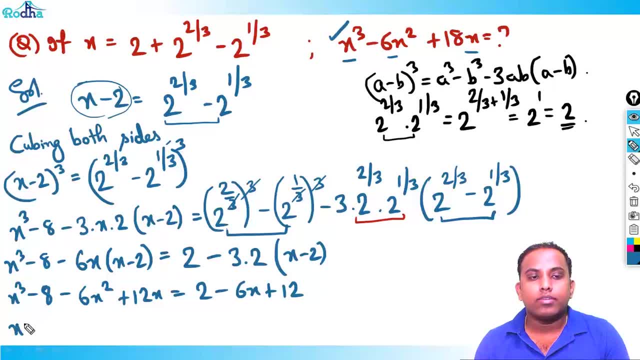 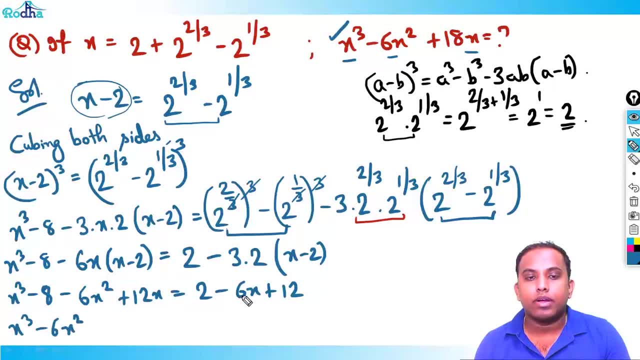 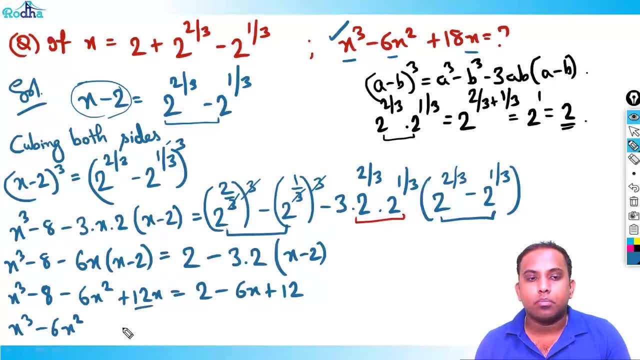 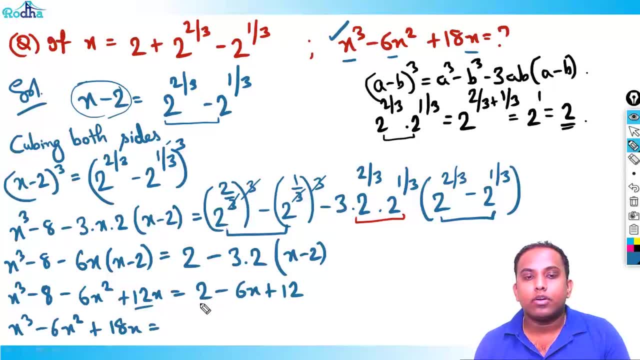 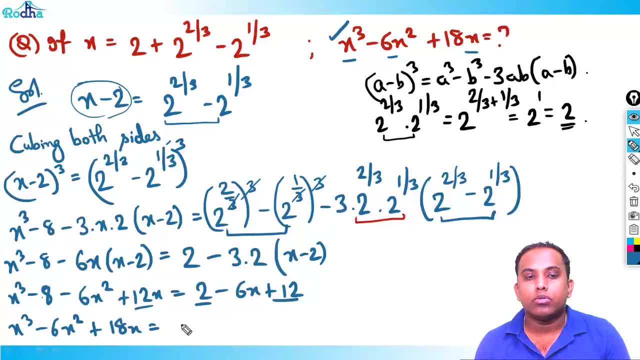 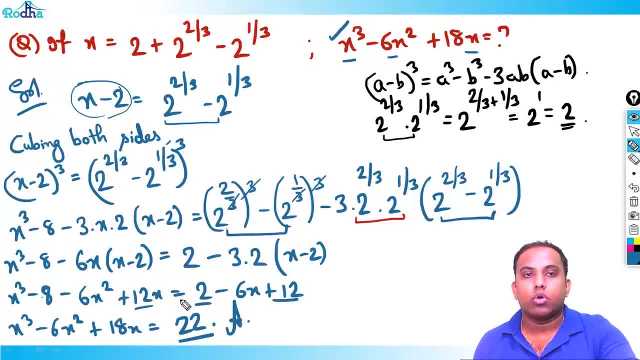 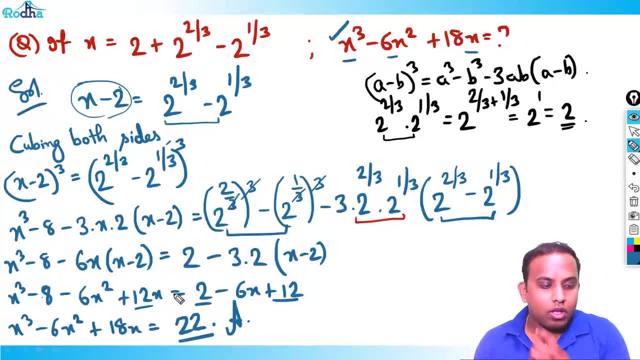 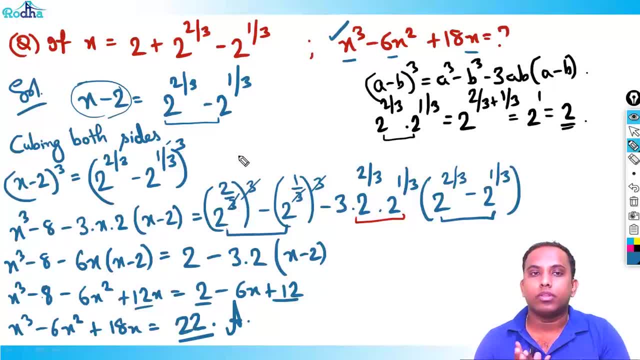 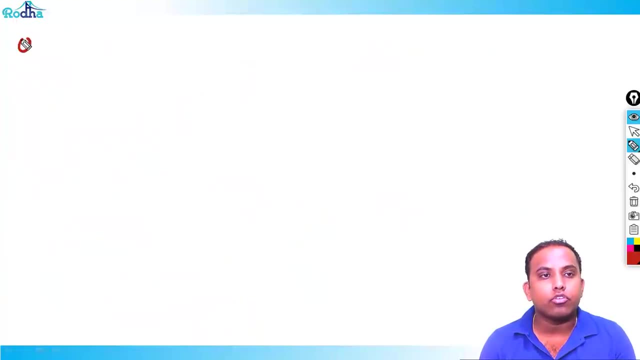 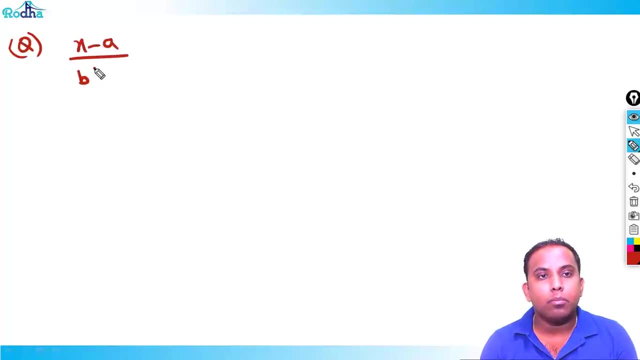 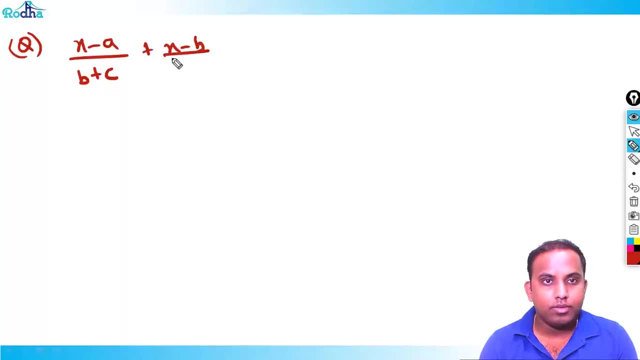 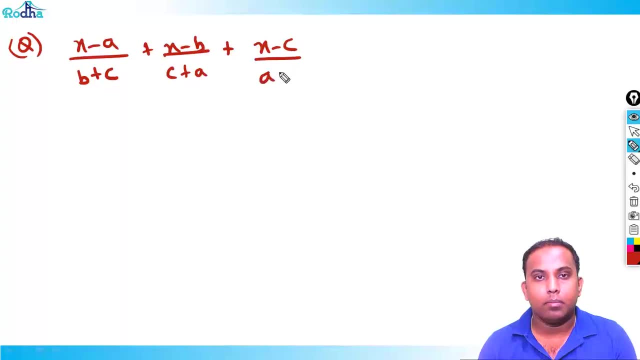 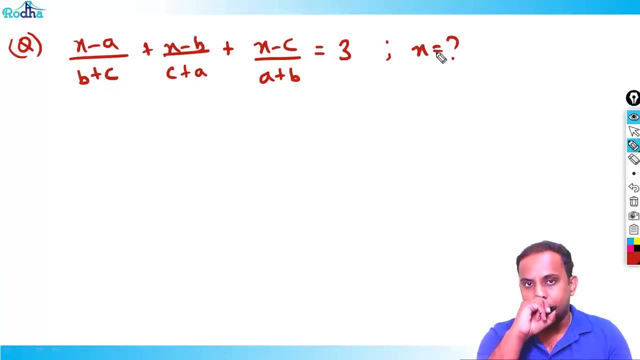 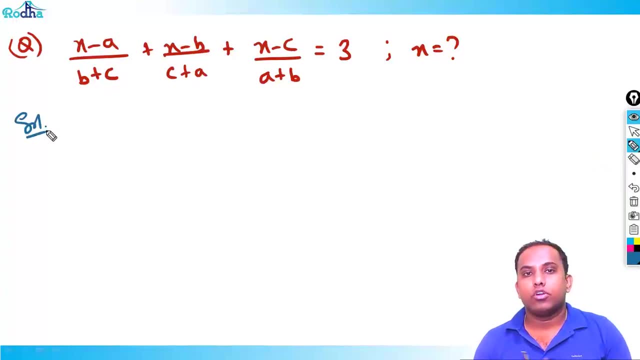 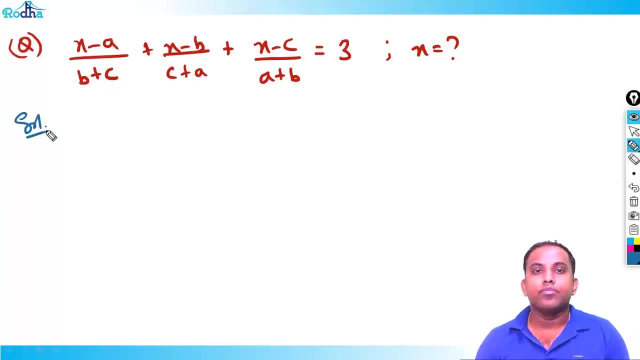 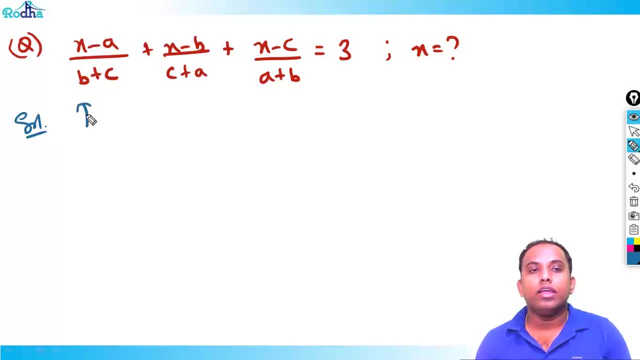 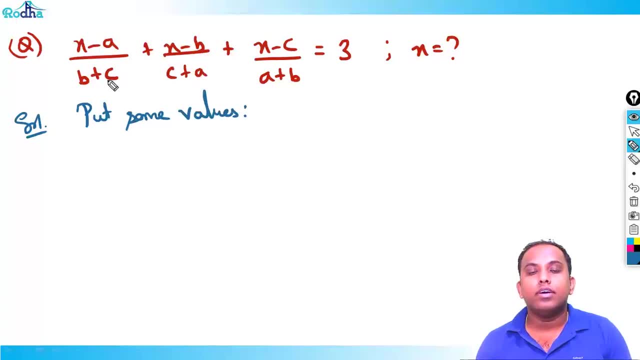 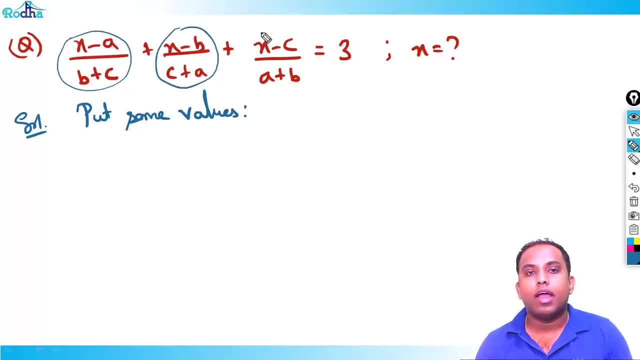 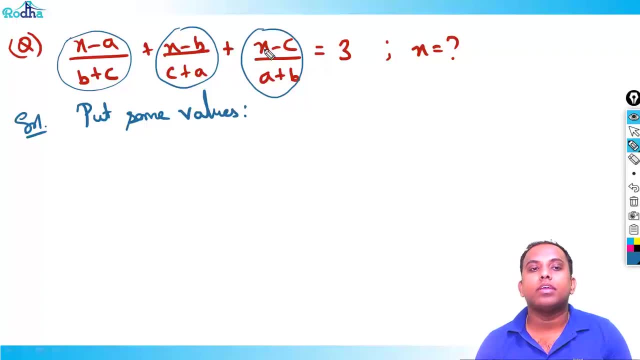 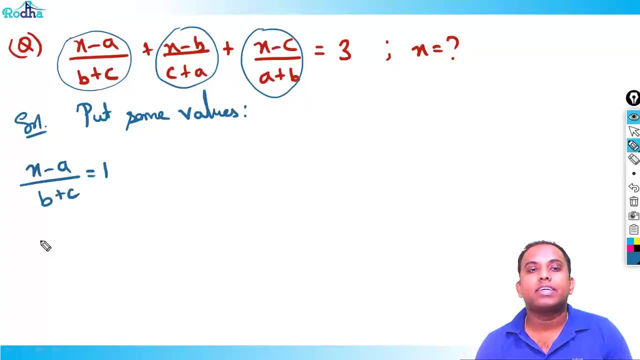 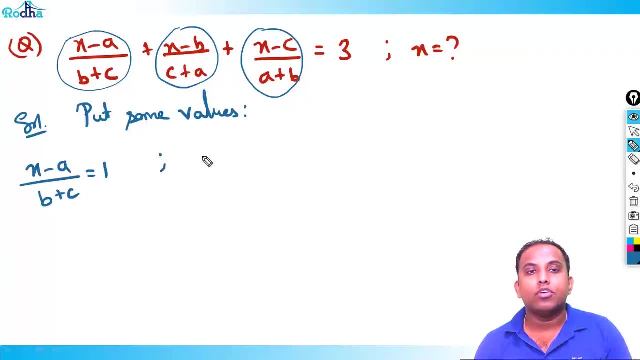 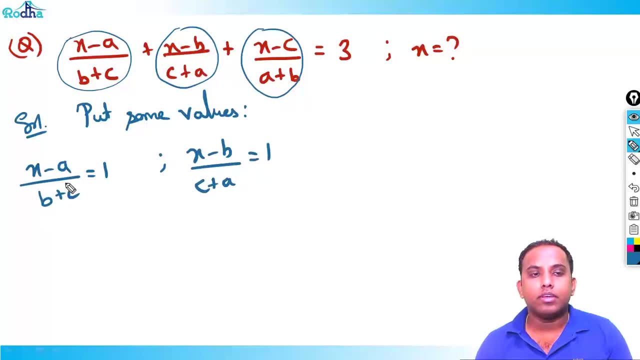 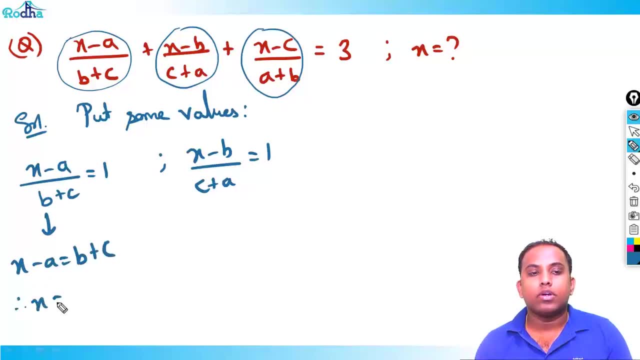 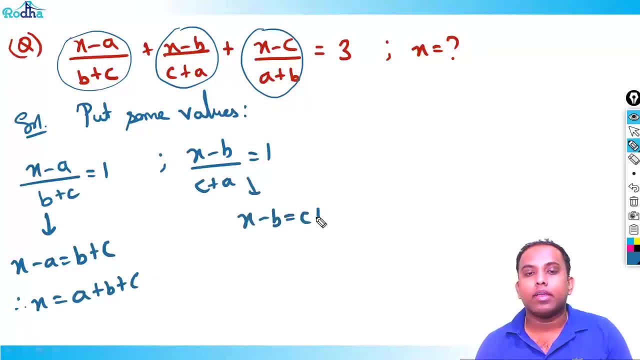 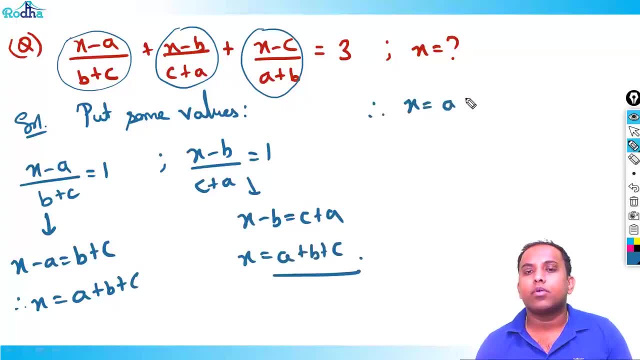 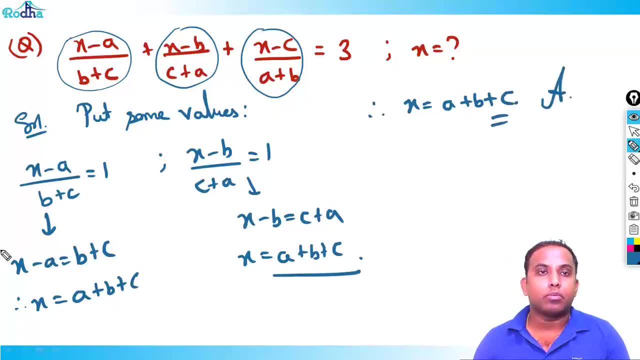 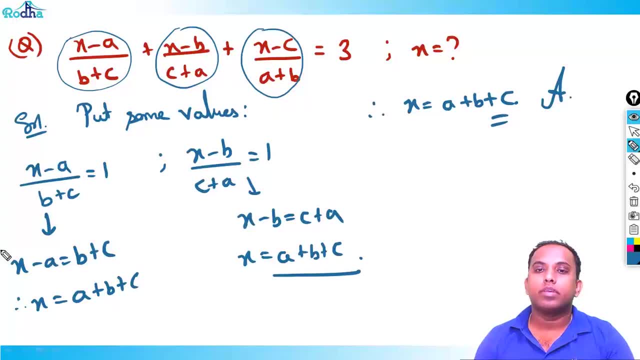 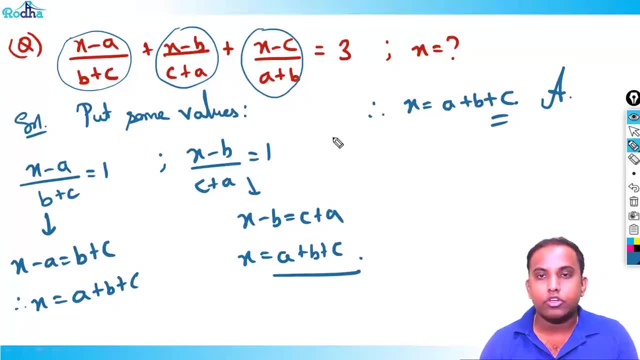 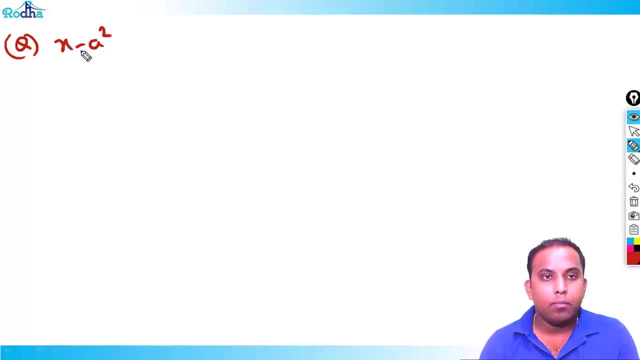 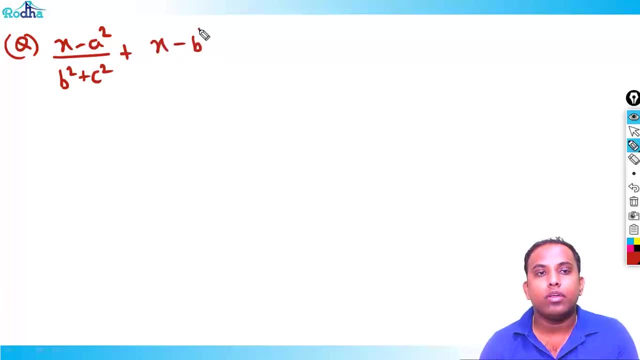 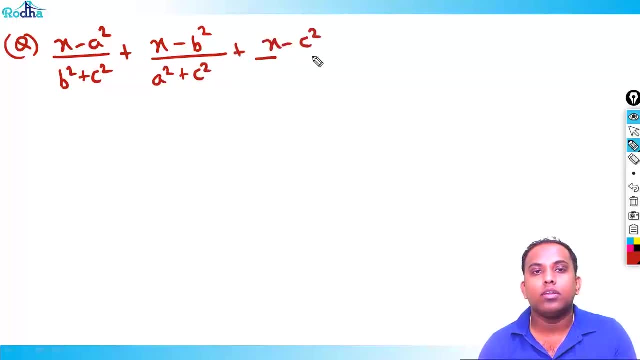 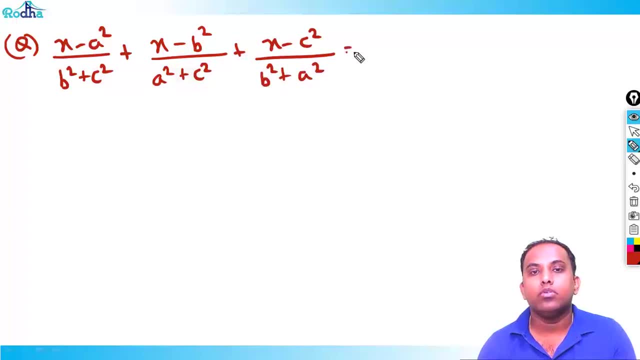 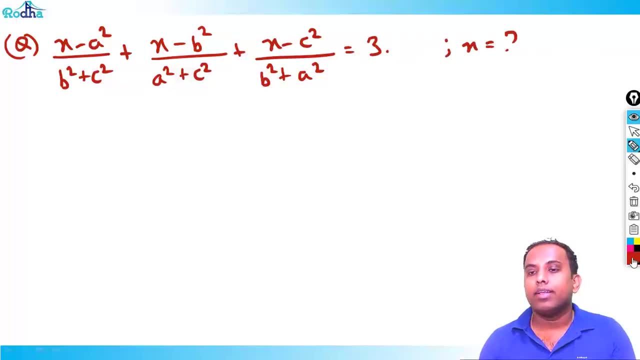 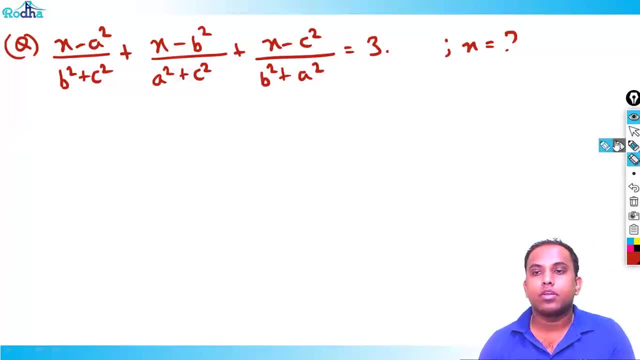 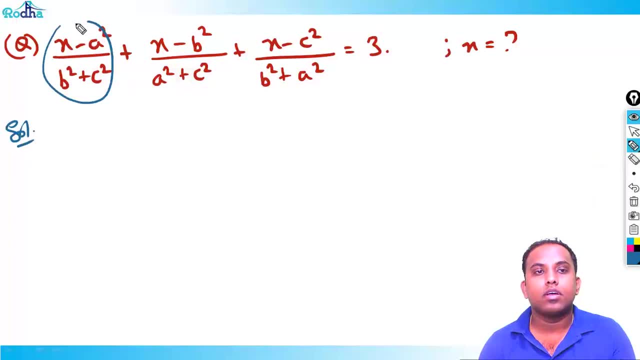 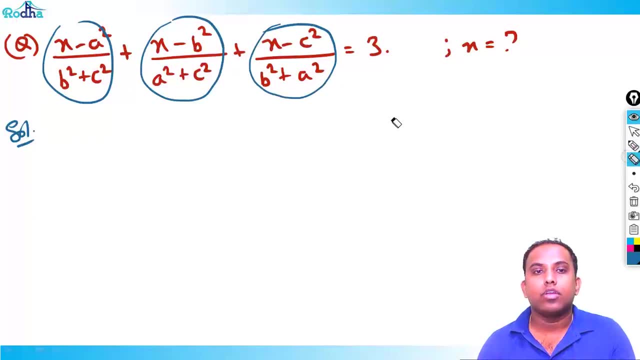 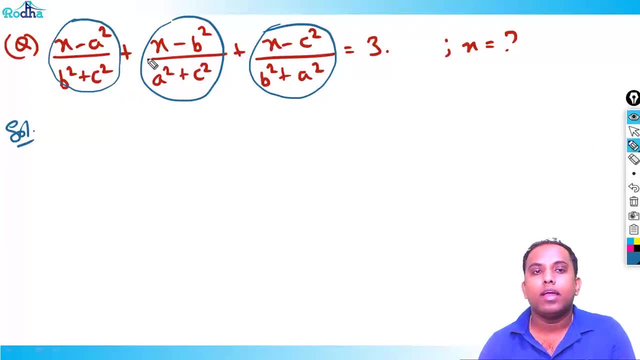 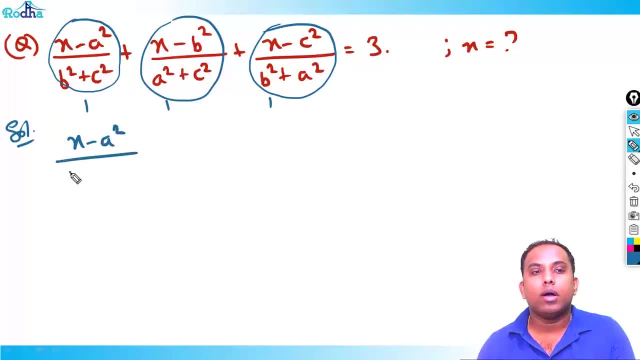 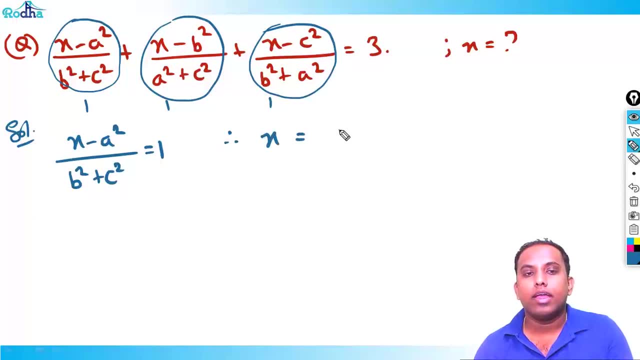 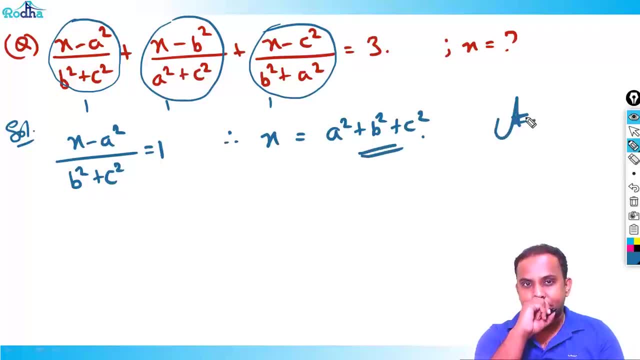 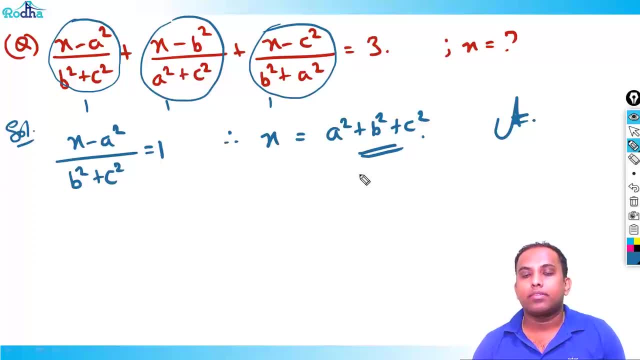 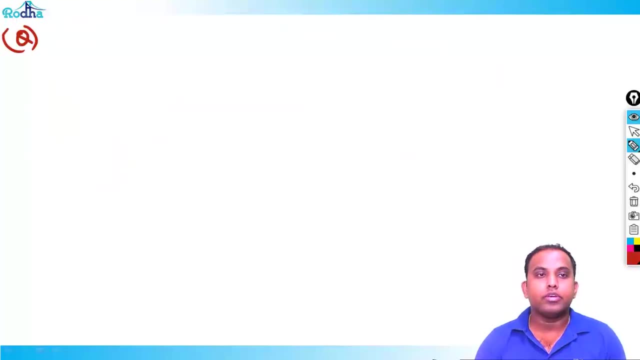 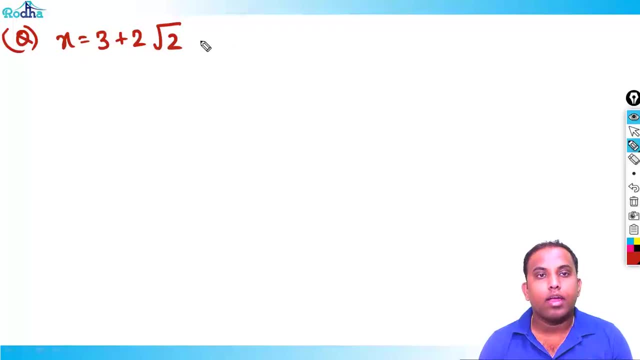 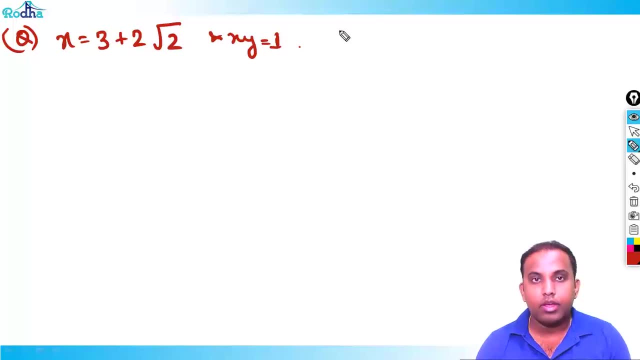 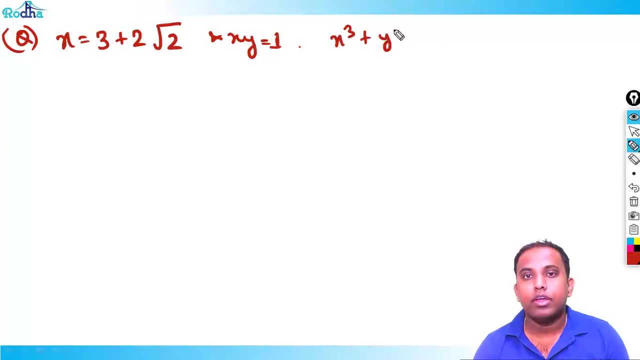 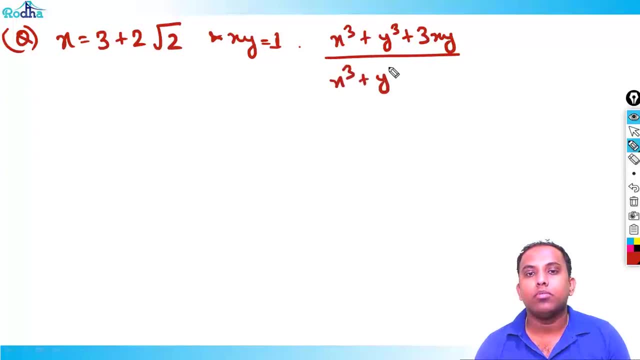 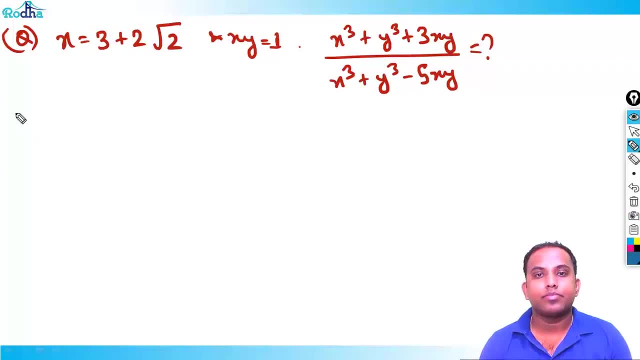 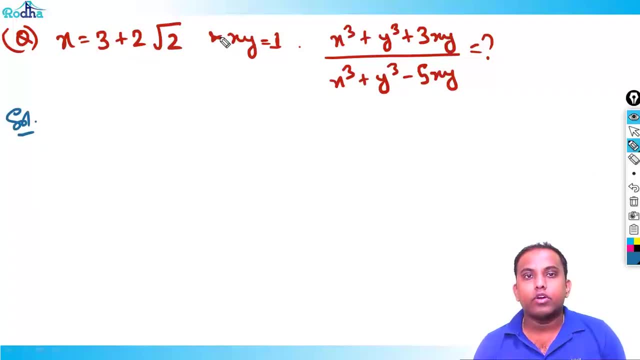 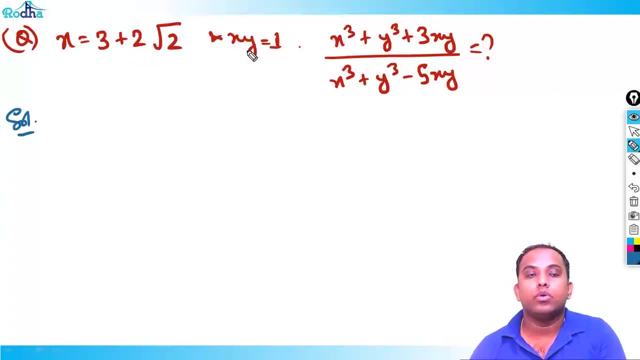 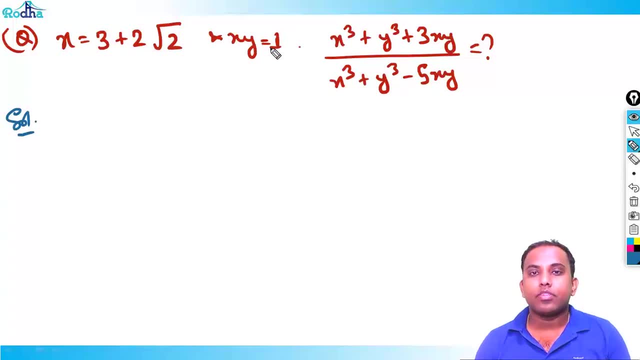 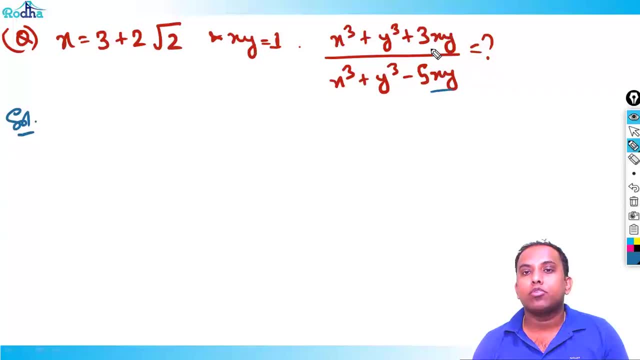 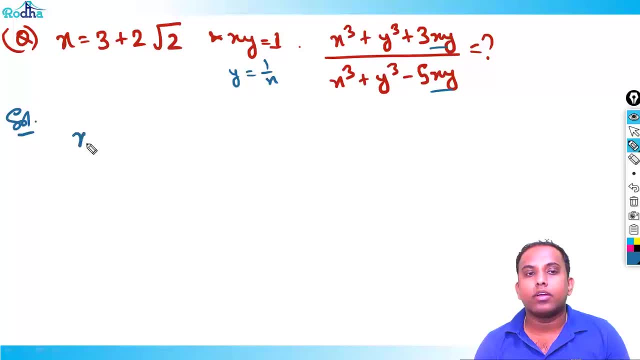 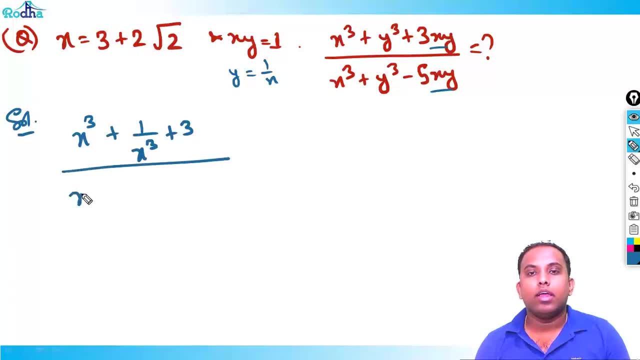 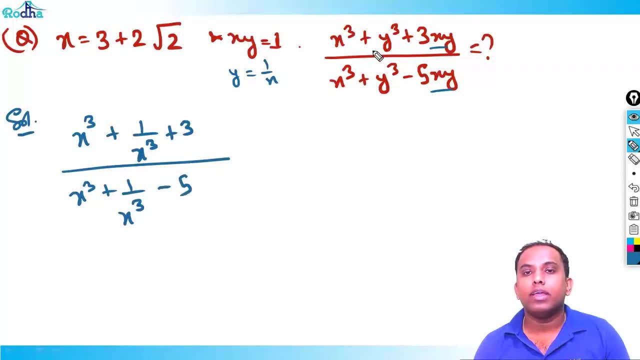 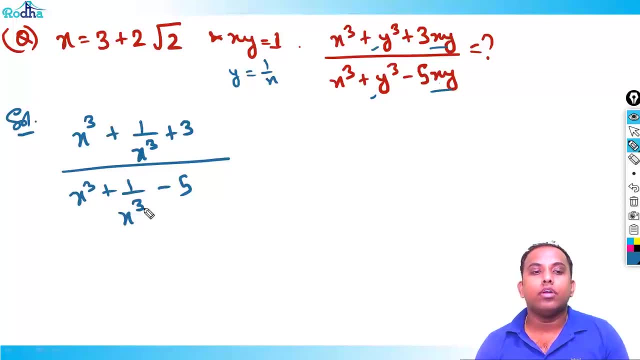 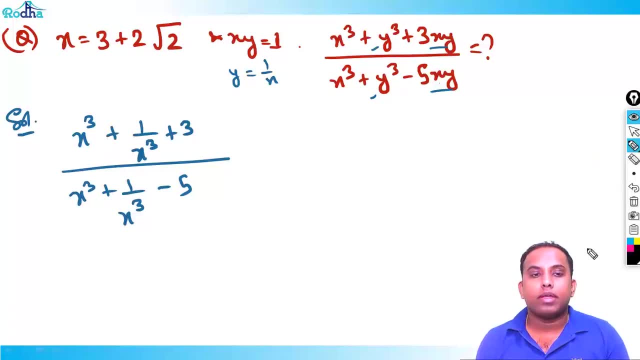 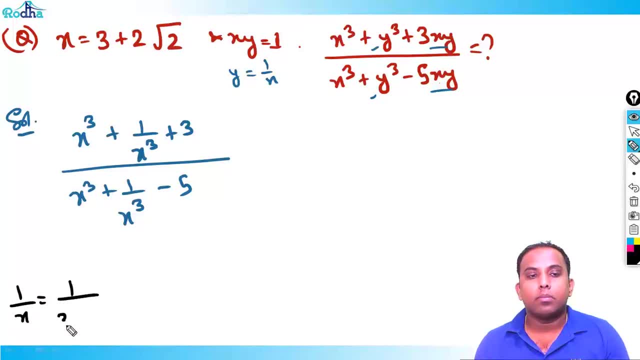 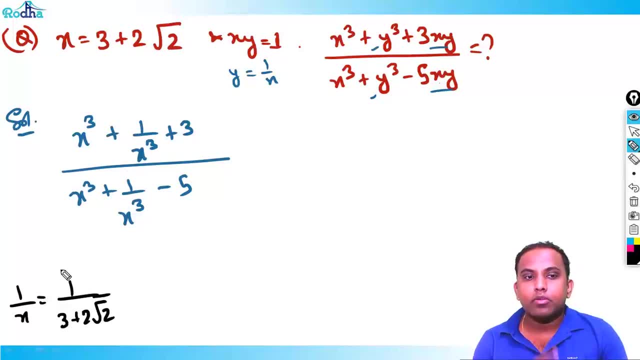 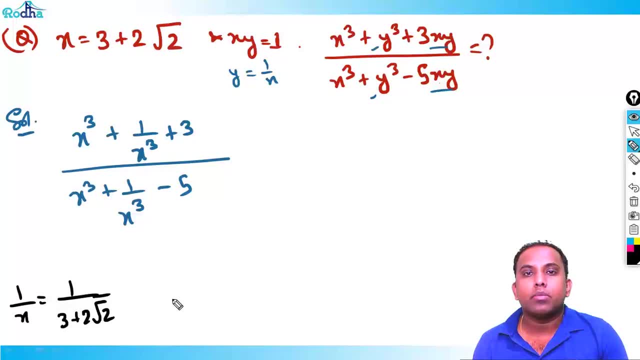 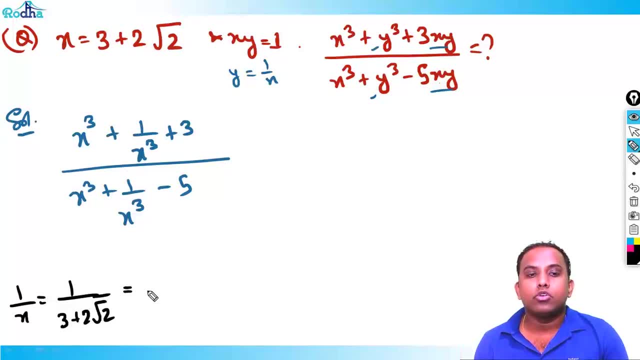 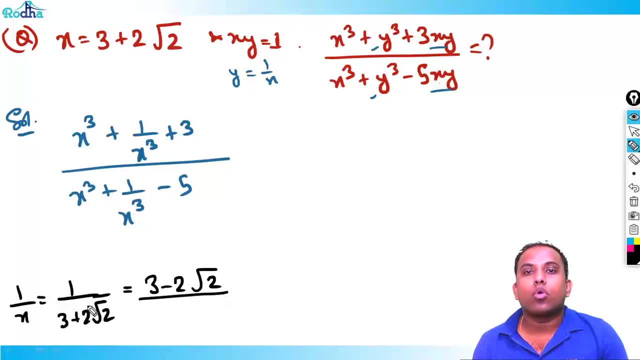 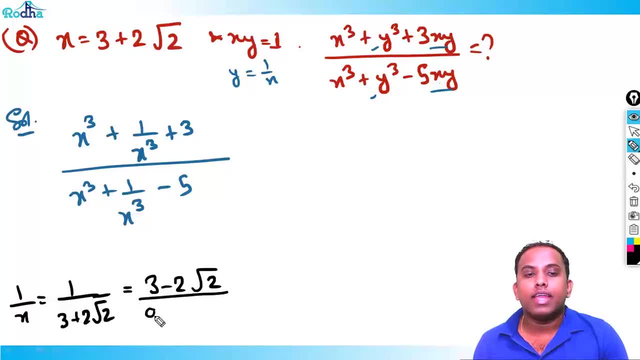 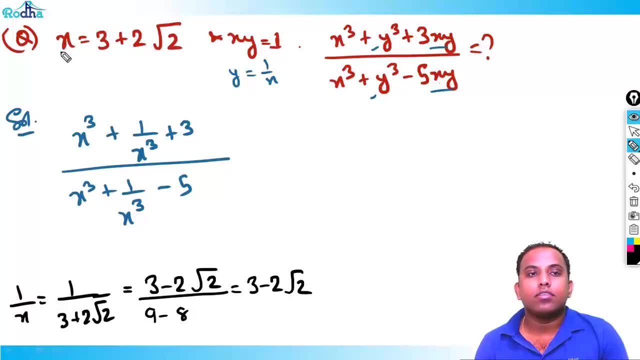 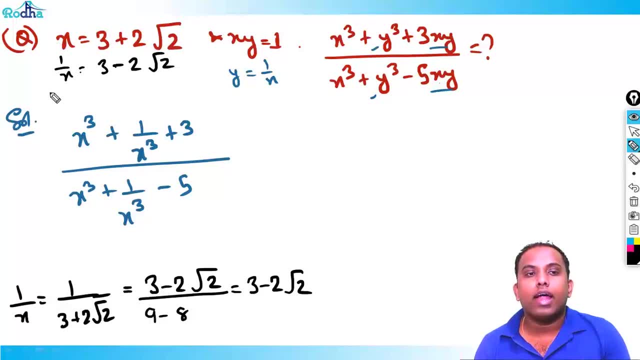 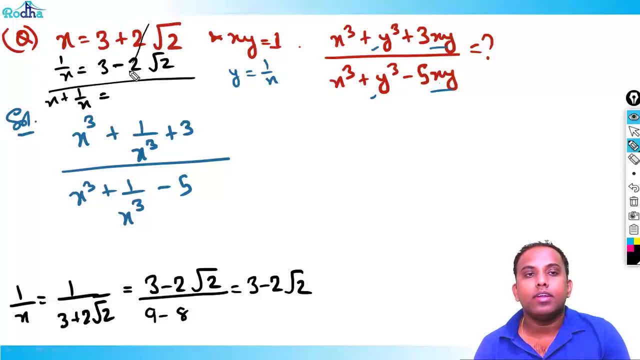 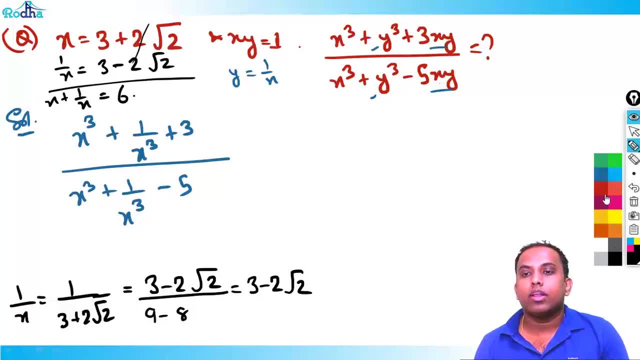 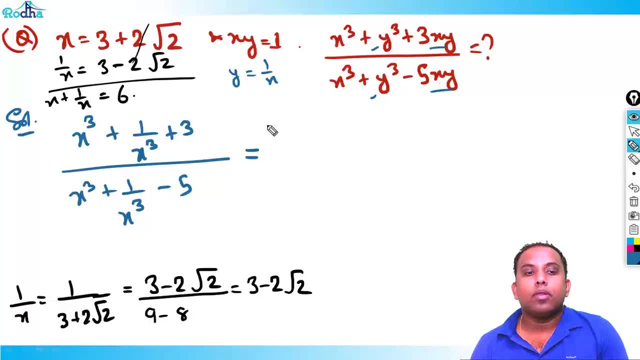 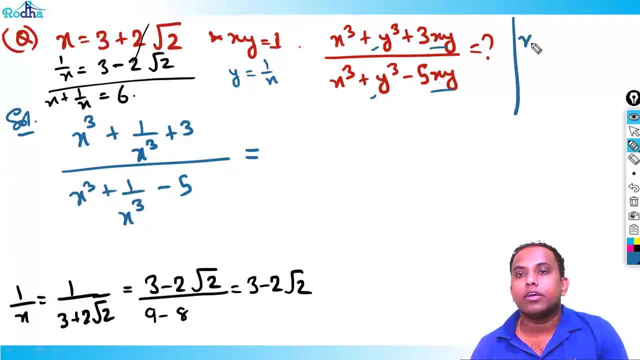 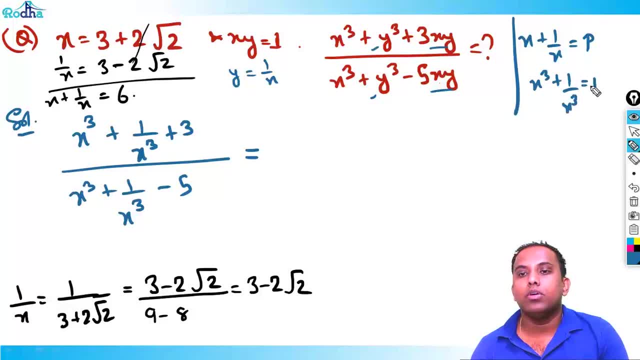